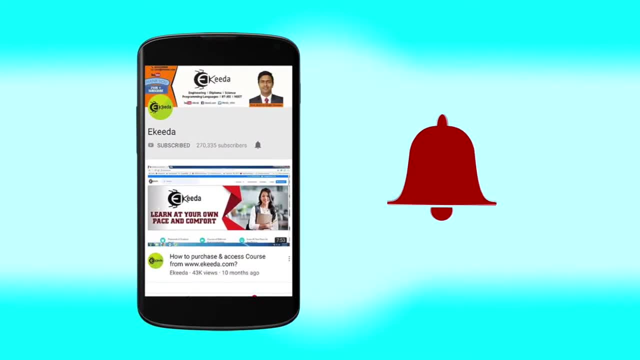 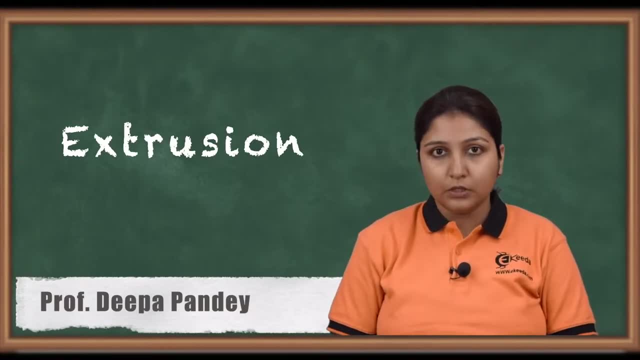 Click the bell icon to get latest videos from eKIDA. Hello friends, today we are going to see a different forming process, which is known as extrusion process, How it takes place and how it is done we are going to see in this video. 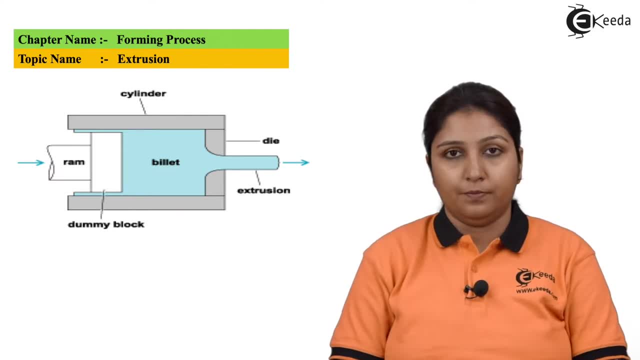 So extrusion can be easily explained by this picture. So in this picture you can see that there is a cylinder. Also there is a billet in which the material is being stored. Also there is a ram and there is a opening. The ram is pushing your billet so that the material comes. 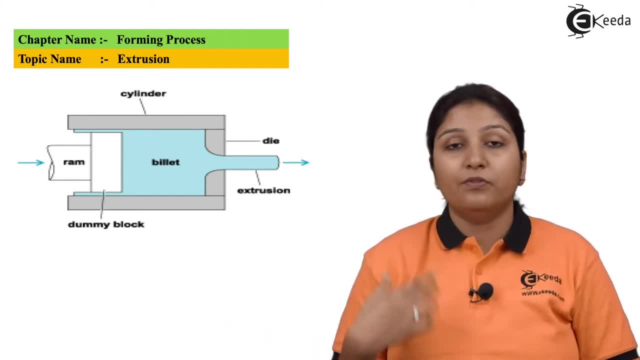 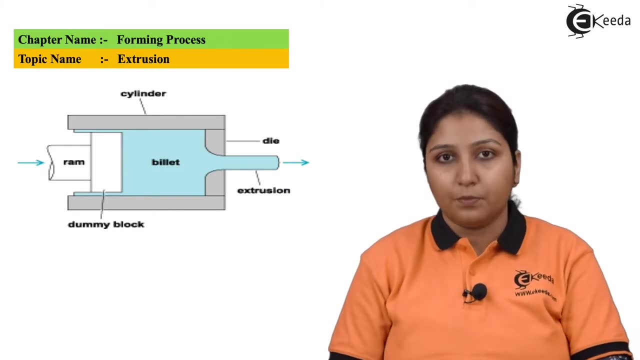 out from the opening and the material comes out in the form of a rod or any kind of hollow object when a hollow part is used. This is your exact extrusion process. So in extrusion material is extracted or material comes out in the form of a rod or in the form of a pipe through a opening, by the action of push or 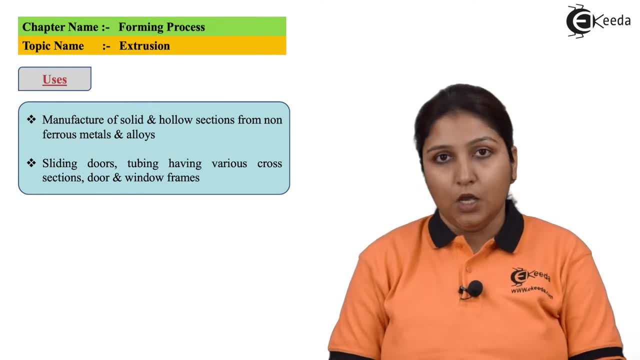 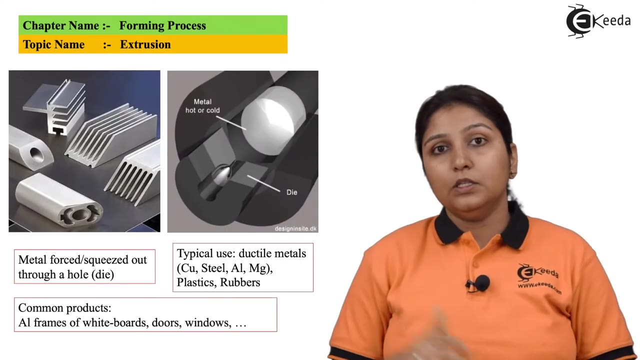 by the action of pull. So what else uses? You can make easily solids or any kind of hollow object through any kind of material like steel, aluminium etc. You can also make sliding doors or any kind of pipes through extrusion process. So in this diagram you can see there are some extruded. 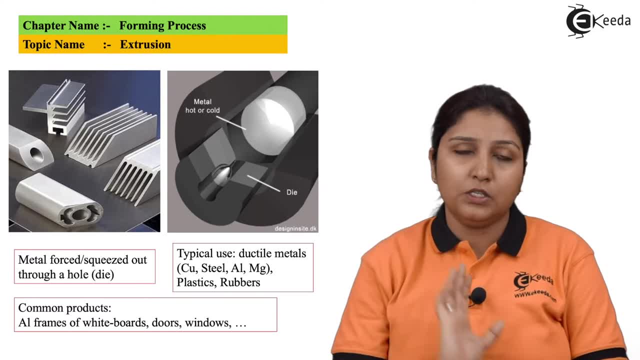 products. Material can be any. It can be any kind of material. It can be any kind of material. It can be aluminium, steel or any other kind of material which can be extruded, But the speciality is material should be ductile. So in this short video you can see that material is coming out. 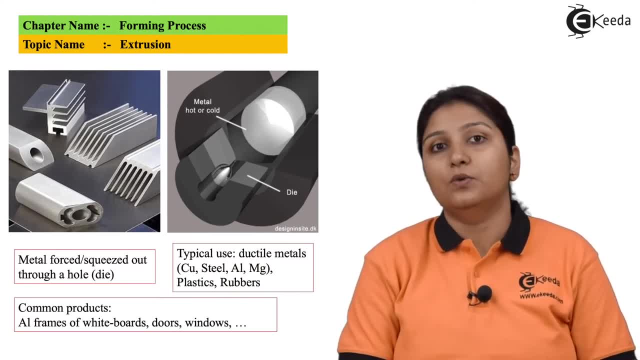 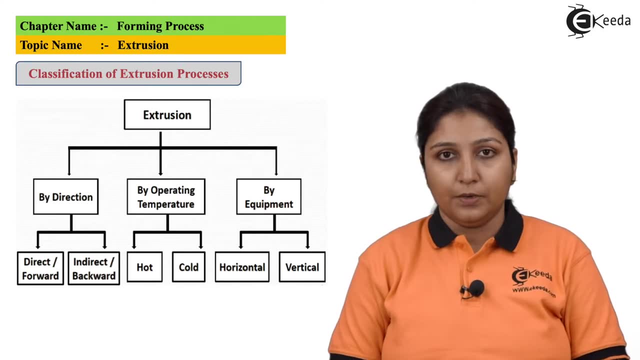 from a small opening which is your extruded products. So in this way extrusion takes place. So this is general classification of extrusion. It can be through direction, It can be through temperature or it can be through equipment. According to the direction, it is classified as direct or indirect extrusion. 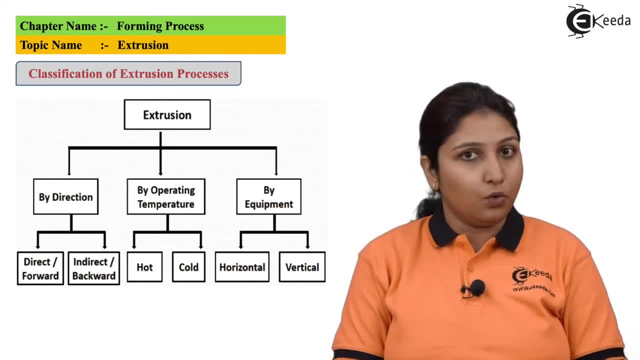 According to the temperature it is classified as hot or cold and according to the equipment it is classified as horizontal or vertical. So these are general classification of extrusion and how it has taken place we have seen in our video. Thank you for watching this video.